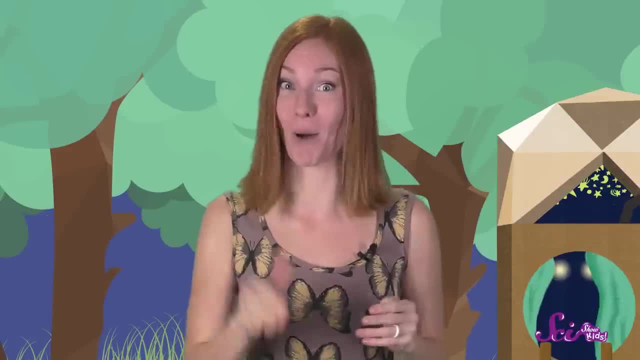 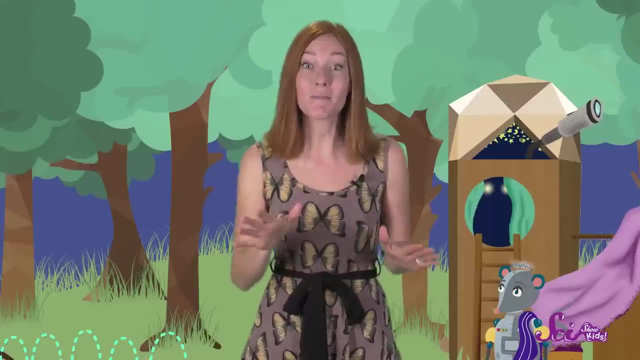 And in the same way, a water slide will only work if you jump onto it. So slipperiness happens when two things touch, And when two things touch they rub against each other. Sometimes those things will slide around against one another like the wet bar of soap against. 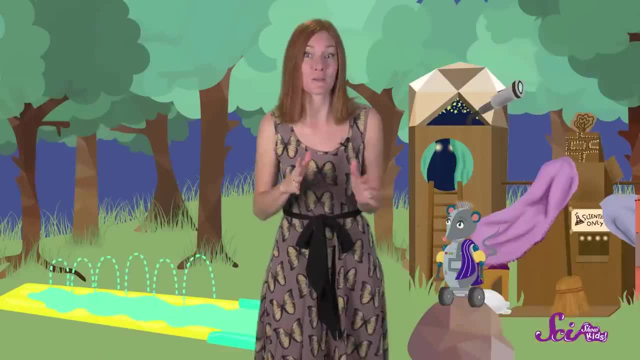 your hand or your body on the water slide, But other times they don't. Sometimes two things that are touching each other will rub against each other. Sometimes, two things that are touching each other will rub against each other. Sometimes, two things that are touching actually keep each other from sliding. 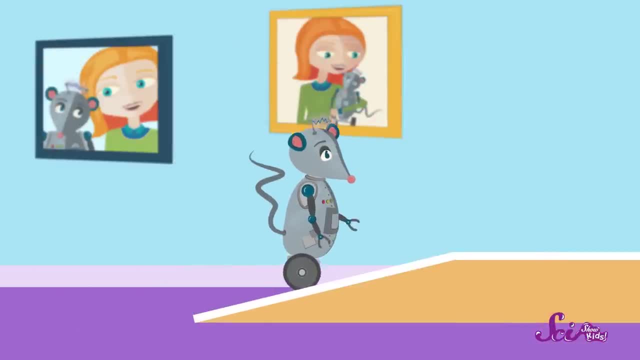 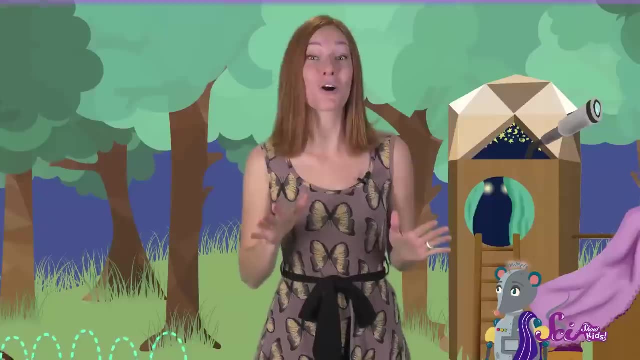 Can you think of some things that aren't slippery? Well, Squeaks can drive up his ramp without sliding back down, and I can sit on my chair without falling out. What makes these things not slippery? It's called friction. Friction is a force between two surfaces that are trying to slide against each other. 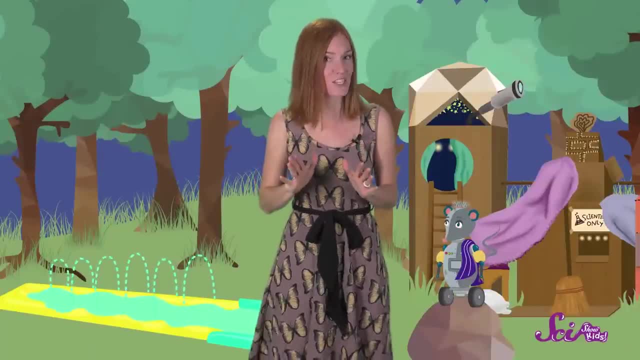 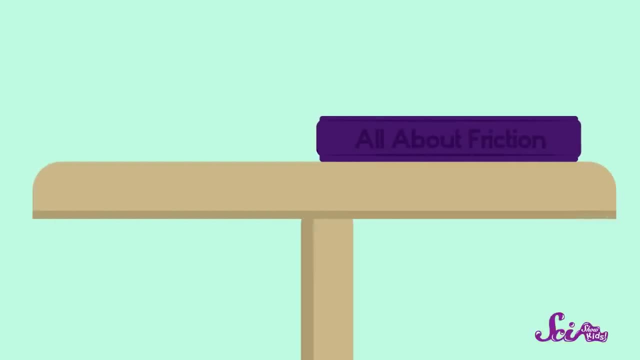 The more friction there is, the harder it is to get those two surfaces to move across each other. Take a book and push it across a tabletop. It's not hard to move, is it? What if you took that same book outside and pushed it on the sidewalk? 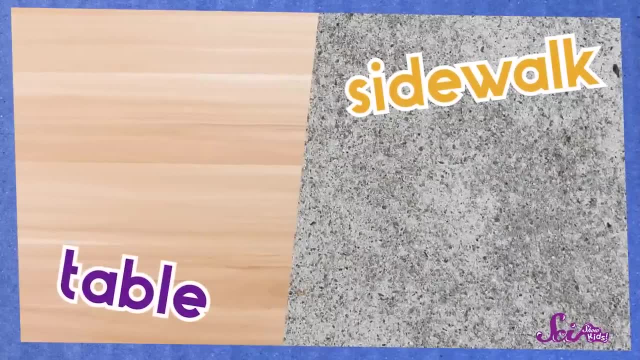 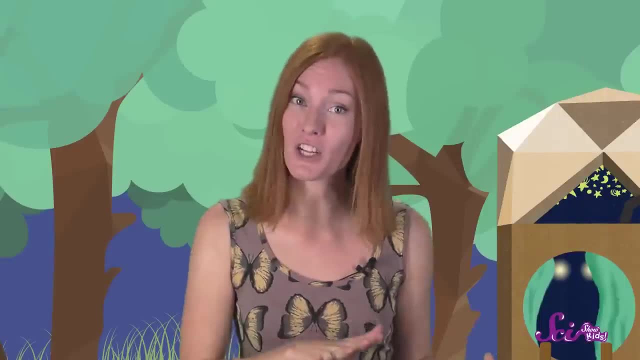 Would it move as easily? Probably not. That's because the sidewalk is rougher than the tabletop and that rough surface creates more friction when the book moves across it. So how much friction there is between two things depends on what kinds of surfaces they 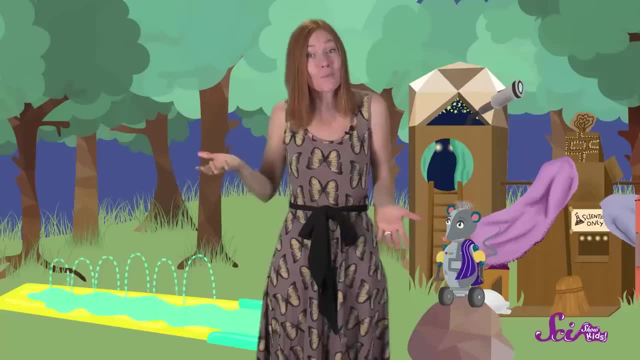 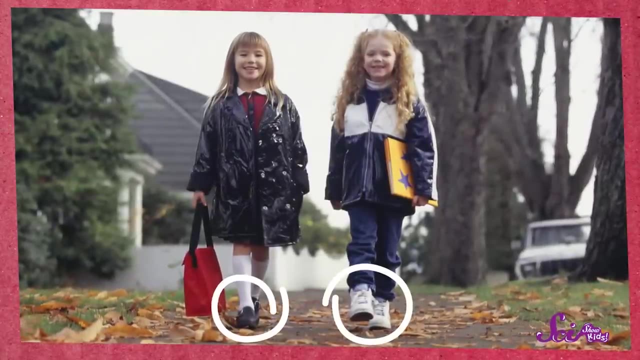 have. Here's another example. Think about when you're just walking around. Normally you're not slipping and sliding all over the place when you walk down the street. That's because there's lots of friction between the bottoms of your shoes and the 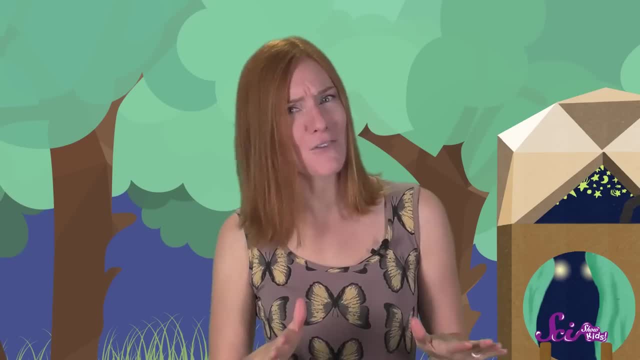 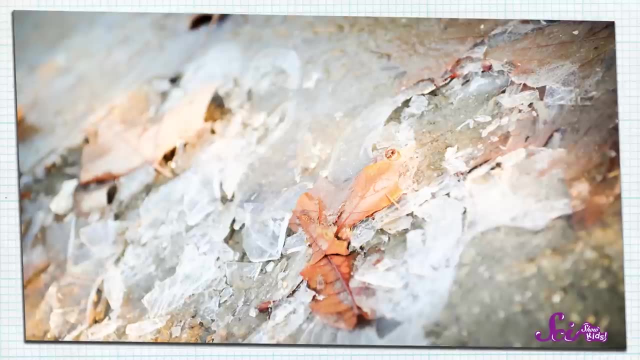 sidewalk. That friction keeps you from sliding. But have you ever stepped on a patch of ice? It can be really slippery. That's because the ice is super smooth, so it creates less friction than the regular dry pavement does. So what does all of this tell us? 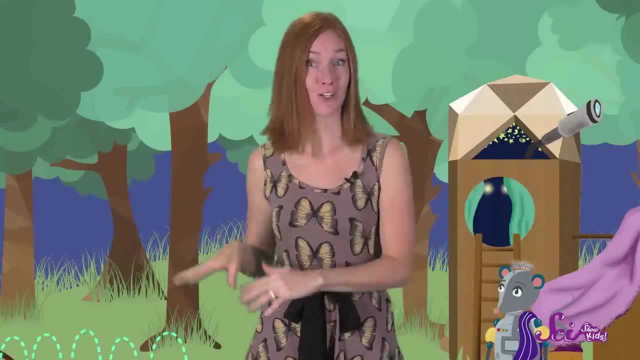 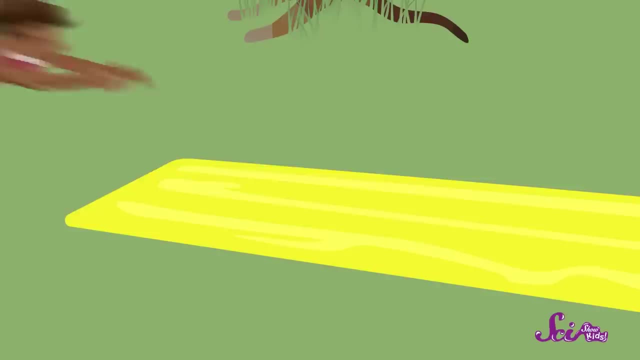 It tells us that things are more slippery when there's less friction. Let's see if that helps us understand how our backyard waterslide works. What do you think would happen if you tried to go down the slide without any water? I don't think you'd be able to slide at all. 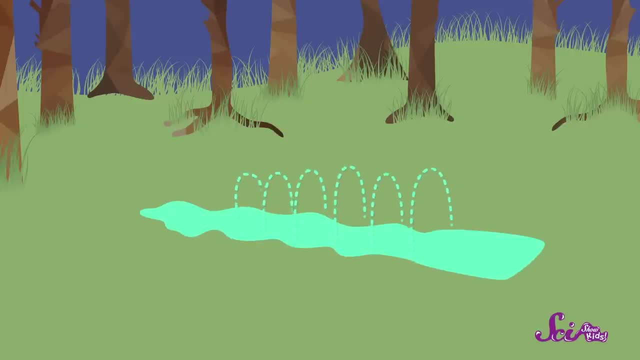 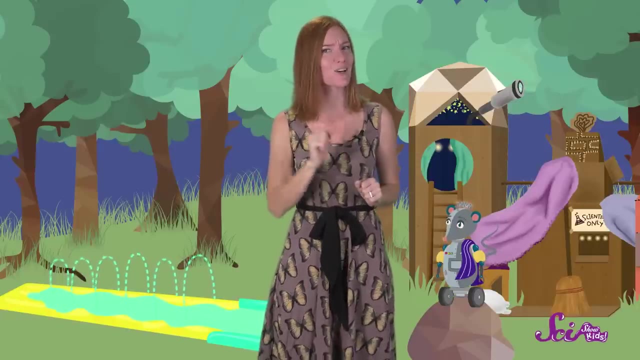 And what do you think would happen if we had a slide? Let's say we have water on the grass but no plastic. I don't think you'd be slipping either. The plastic slide gives you a smoother surface to play on than the grass, so that helps make.